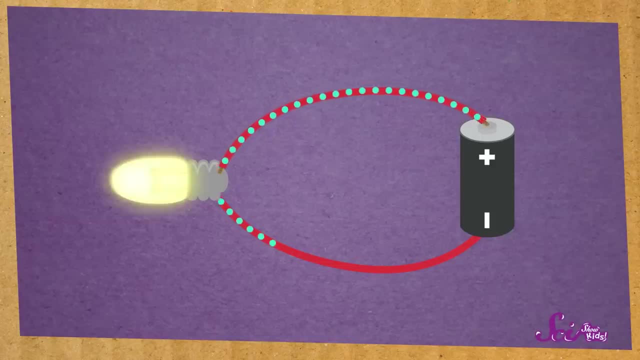 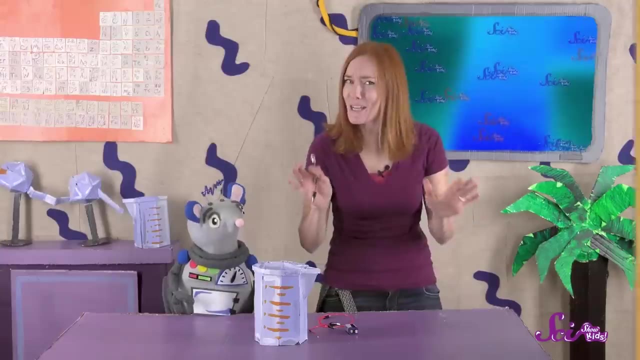 As the electricity goes through the bulb. the bulb lights up, The electricity leaves the bulb and flows back through the battery. Then it follows the circuit all over again. As long as there are no spaces in the circuit, the bulb will stay lit. 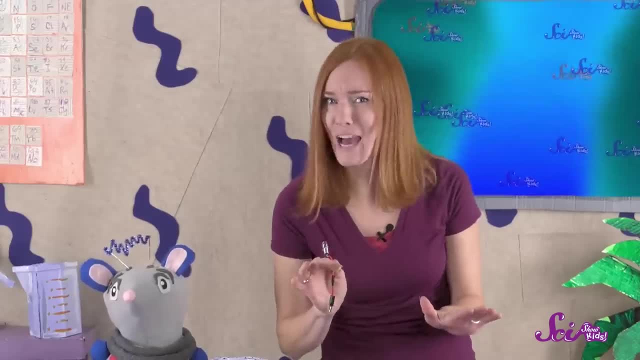 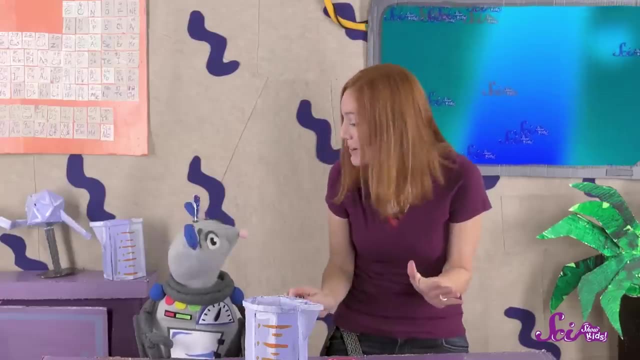 But what if we want to turn the light on and off? Then we have to break the circuit, which means we need to put a space in it somewhere to stop the flow of electricity. So we use a switch. A switch allows us to make a space in the circuit if we want to. 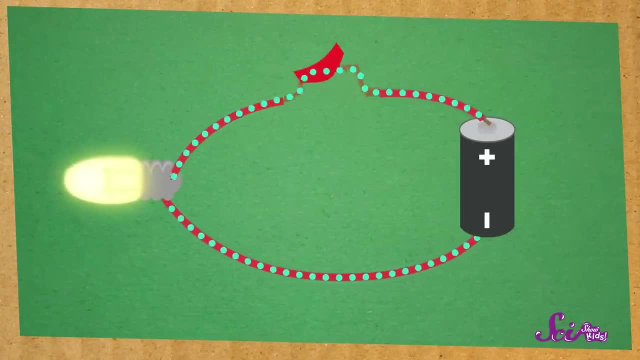 When the switch is on, there's no space in the circuit and the light bulb is lit. But when we move the switch off, we open up a space. The electricity can't jump over the space, so it can't reach the light bulb and the 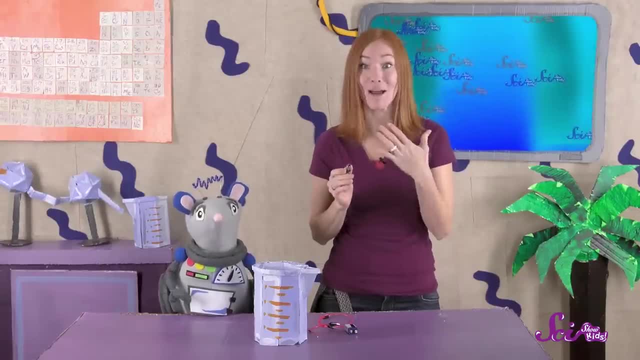 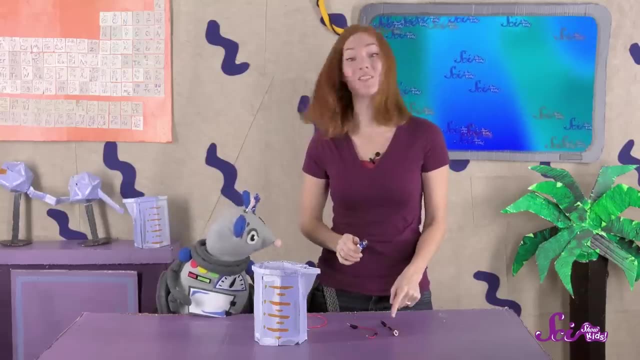 light bulb stays off. OK, so I'm going to try to build my own circuit using some of the parts that I have here. I have a power source, this battery and a wire for the electricity to travel through, and a little light bulb. 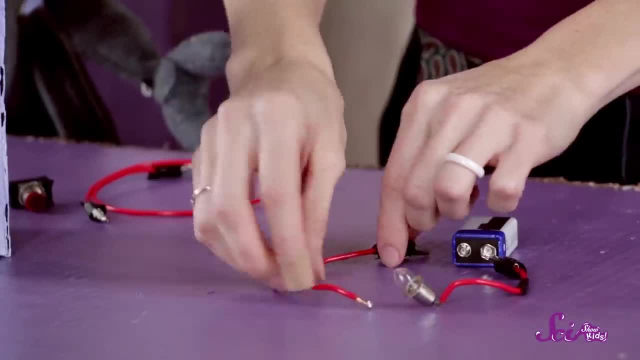 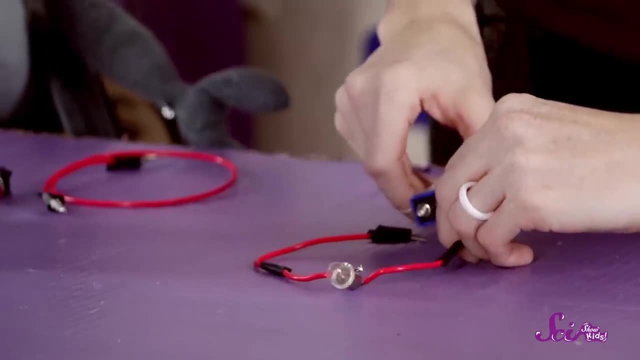 If I arrange everything just so, it kind of looks like a circle, but the bulb isn't on. That's because I haven't connected all of the pieces together. Remember, there can't be any spaces in the circuit. So I'll connect the wires to the power source. then I'll connect one wire to the. 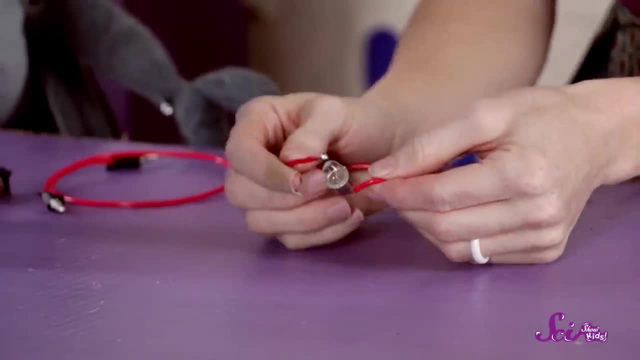 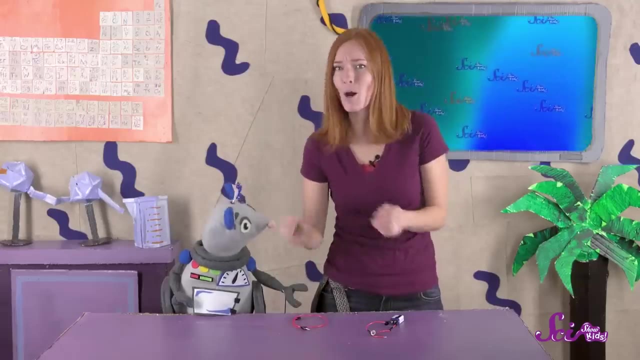 bulb, And when I connect the other wire to the bulb and complete the circuit, the bulb lights up. Now I'm going to add something else to make it work a little more like a flashlight. does I have this part that looks like a button? and I'll put it right here. 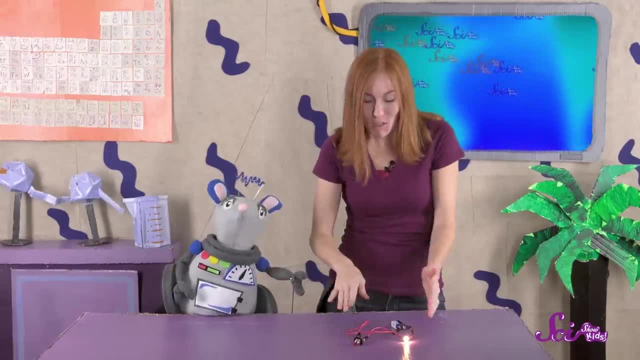 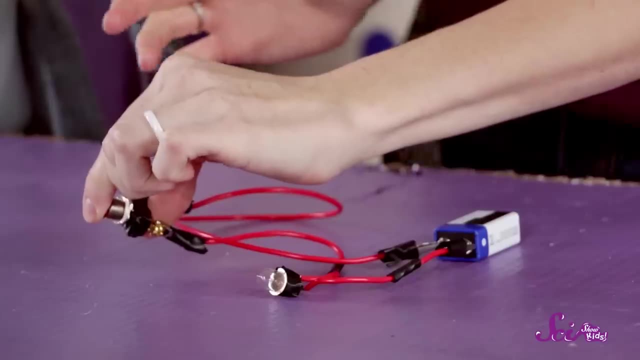 And look, the bulb is lighting up. That means that there are no spaces in the circuit. OK, Squeaks, let's press the button and see what happens. Hey, the light bulb went off. That means, when I press the button, the circuit is incomplete, which means that I've created. 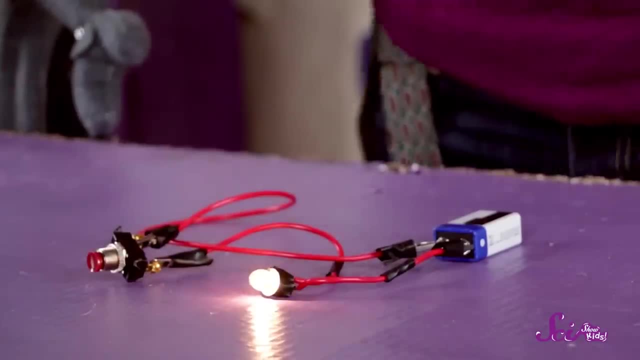 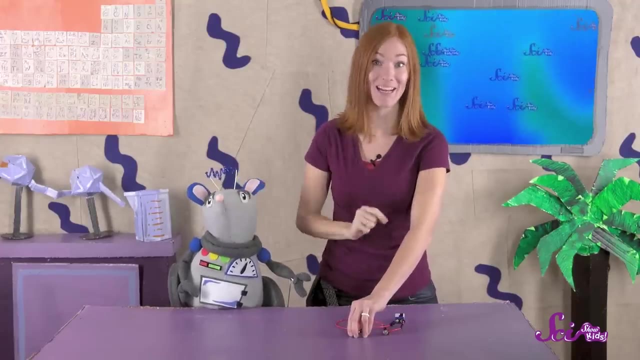 a space And when I let go of the button the circuit is complete again. When I press the button, the electricity from the battery can't cross the space, so it can't get to the bulb and make it light up. The button is a switch, kind of like the switch on a flashlight.